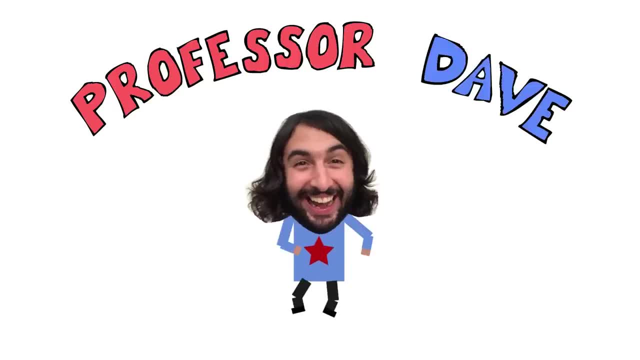 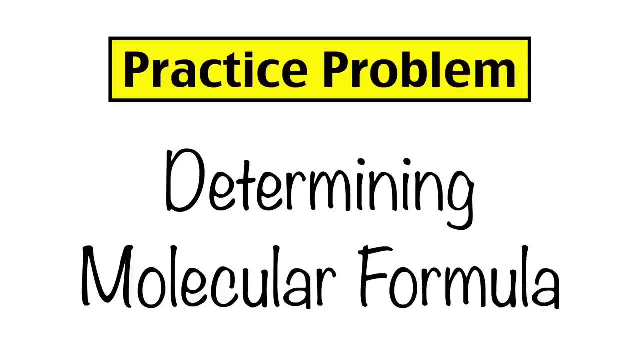 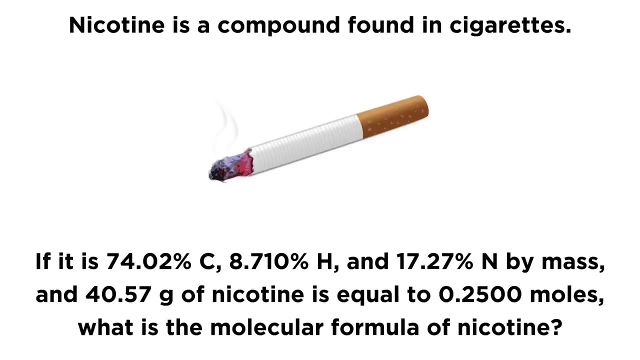 He knows a lot about the science stuff. Professor Dave Explains Today. let's get some practice on determining molecular formula. So let's take a look at the question. nicotine is a compound found in cigarettes. If nicotine is 74.02% carbon, 8.710% hydrogen and 17.27% nitrogen by mass and 40.57 grams of nicotine, 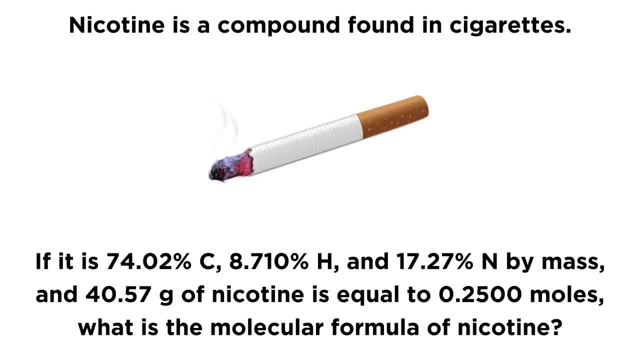 is equal to 0.2500 moles. What is the molecular formula of nicotine? So, if you're not sure how to get this going, go ahead and check out my tutorial on elemental analysis. That is going to give you the strategy you need. 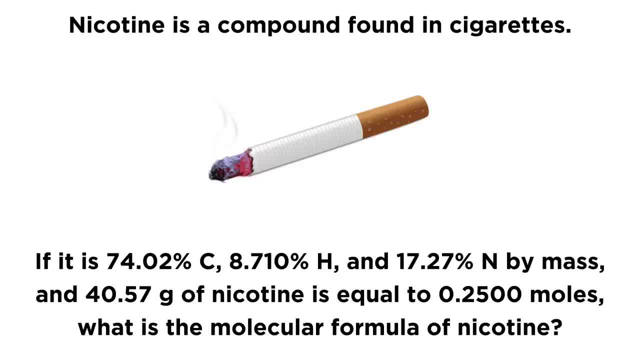 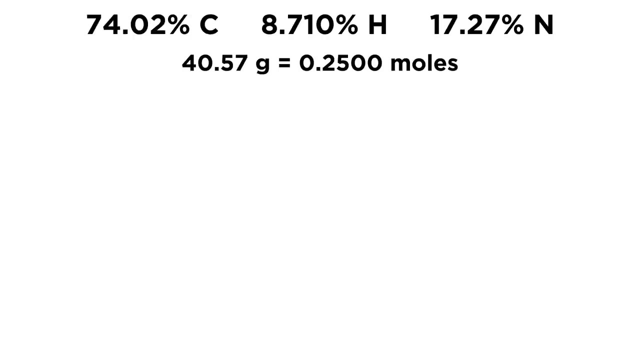 To answer this question and when you're ready, go ahead and give it a shot. So we have our mass percentages up at the top here and we also have our information that tells us that 40.57 grams of nicotine is equal to 0.2500 moles. 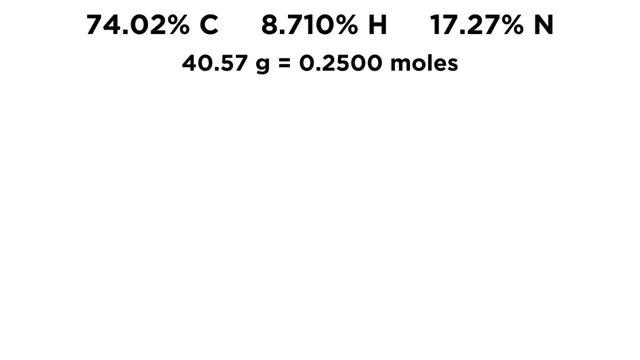 So what are we going to do with this information? Well, the easiest way to do this is to go ahead and assume some mass of nicotine to start doing some calculations, Since it's totally arbitrary what mass we choose, because we're dealing with percentages. let's just use 100 grams and make 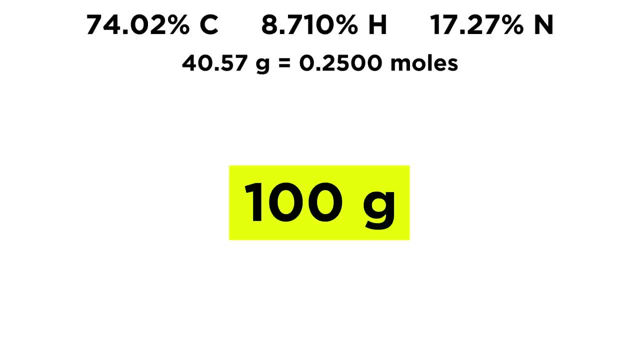 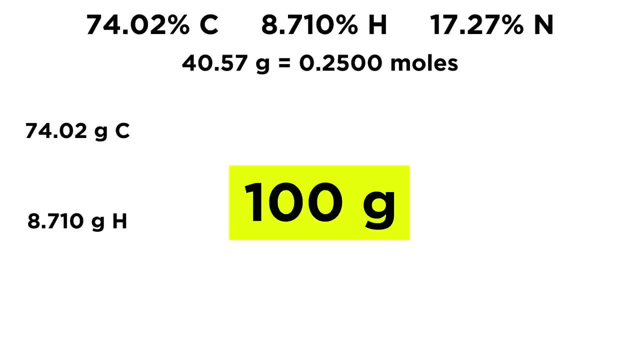 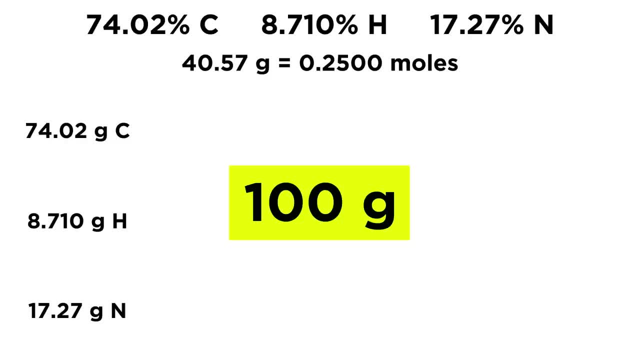 which are out of 100, and turning them into grams. Now we need to convert these into moles, because masses don't tell us anything. Whenever we are doing calculations of this nature, we always want moles. So let's take our mass of carbon. 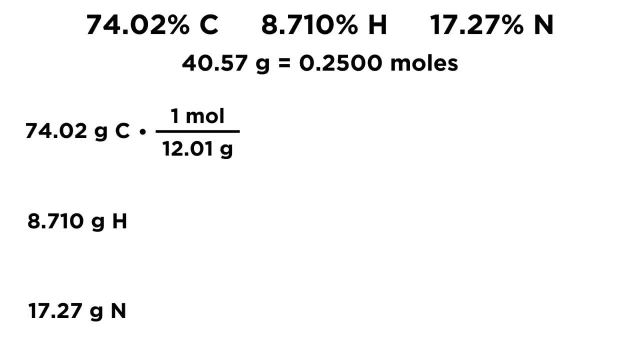 and multiply by 1 mole over 12.01 grams, That is the atomic mass of carbon. Grams will cancel and we have 6.163 moles of carbon in our hypothetical sample of nicotine. Now for hydrogen. let's multiply by 1 mole over 1.008 grams. That is the atomic mass of hydrogen. 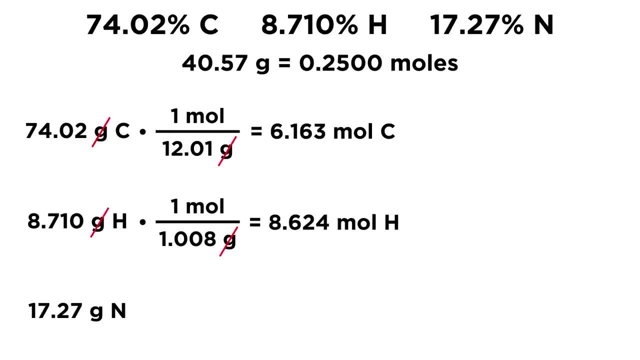 Grams will cancel and we have 8.624 moles of hydrogen. Lastly, for nitrogen, we multiply by 1 mole over 14.01 grams, That's the atomic mass of nitrogen. Grams will cancel and we have 1 mole over 14.01 grams. 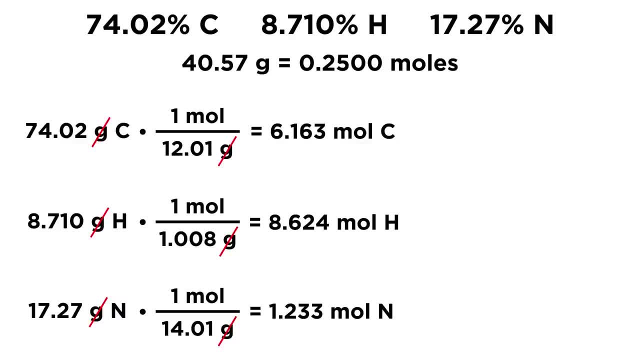 Grams will cancel, and we have 1.233 moles of nitrogen. So in this sample we have this many moles of each of these elements. So this tells us something about the ratio of these elements in the compound. So how can we get this in a way that's a little more? 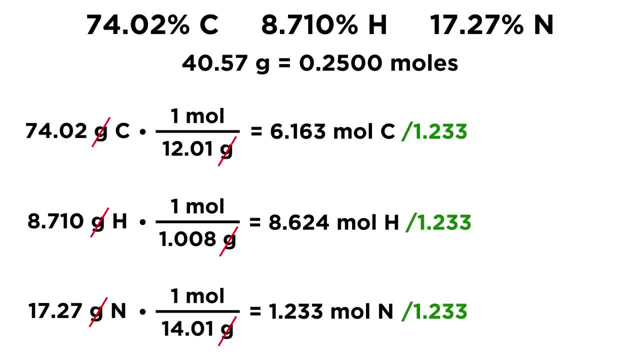 useful. What we can do is divide each of these values by the smallest, so that we get 1 for the smallest one, and then some for the second, And then some ratio for the others, and hopefully they'll turn out to be integers, and that will give us the empirical formula. 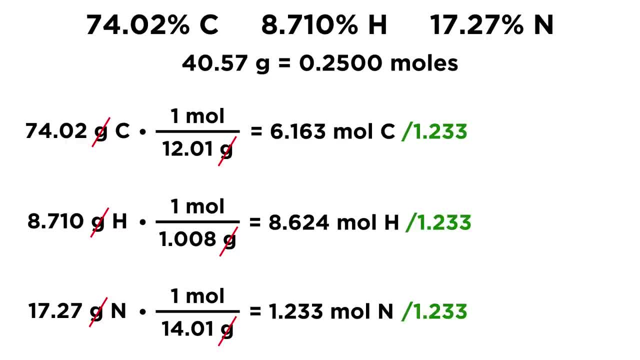 So if we divide each of these by the smallest one of them, which is 1.233,, we end up with 1 mole of nitrogen, and we also end up with integer values for carbon and hydrogen. We have 5 and 7.. 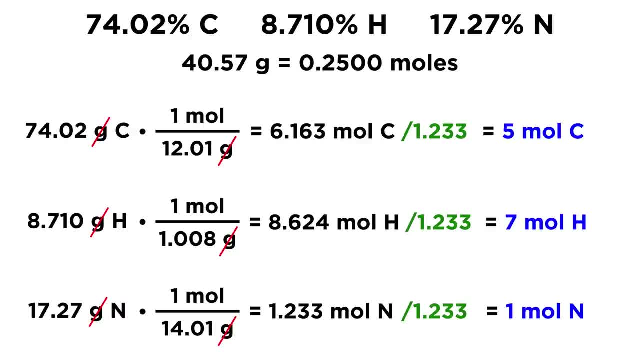 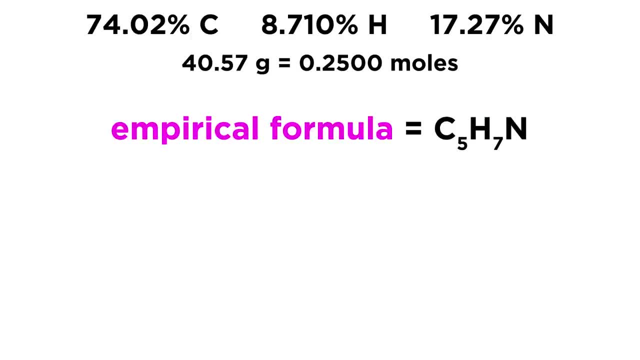 So that means for every nitrogen atom in the sample we have 5 carbon atoms and we have 7 hydrogen atoms. So that means the empirical formula of nicotine must be C5H7N. That is the only way for these mass percentages to work out the way that they are. 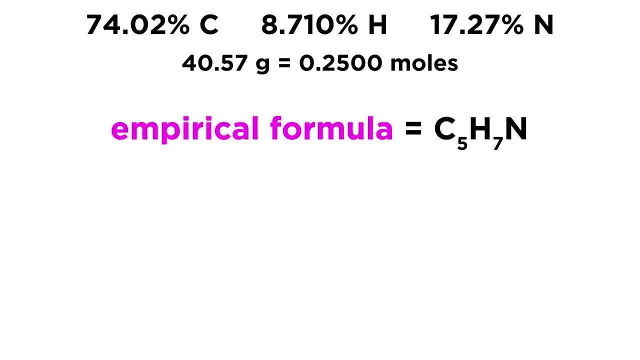 But once again, we need the molecular formula In order to get that, we need the molecular mass or the molar mass. And so let's take this other bit of information we have If we want to know the molar mass of nicotine in grams per mole. well, we have a formula. 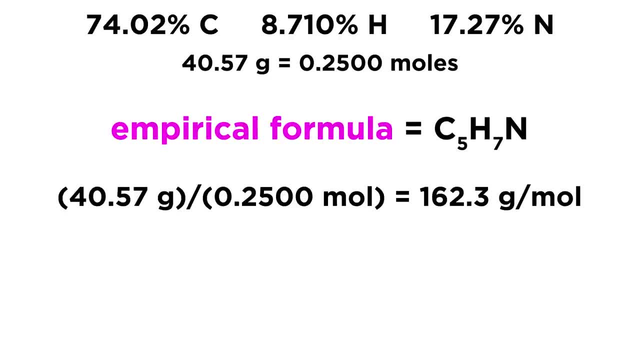 We have 40.57 grams, and we can just divide that by 0.2500 moles, That will give us a value in grams per mole, And so we get 162.3 grams per mole. So how is that useful?